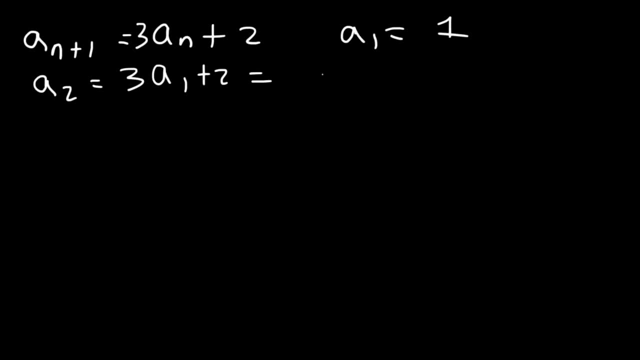 second term is 3 times the value of the first term plus 2.. So it's 3 times 1 plus 2, which is 5.. Now if you want to find the third term, it's 3 times the second term plus 2.. The second term is 5.. 3 times 5 is 15 plus 2 is 17.. Now if we 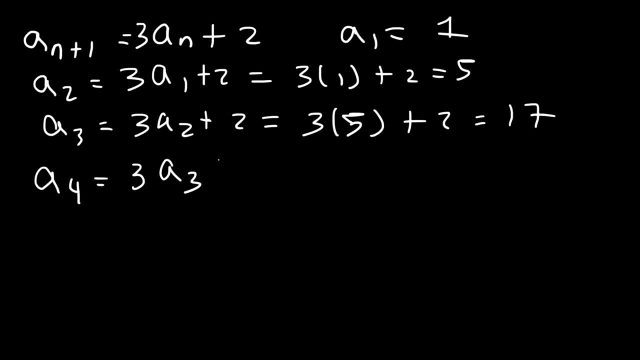 want to find the fourth term. it's 3 times the third term plus 2.. The third term is 17.. 17 times 3 is 51 plus 2, that's 53. So that's the value of the fourth term. Let's try another example. So let's say that a of n is equal to 2. 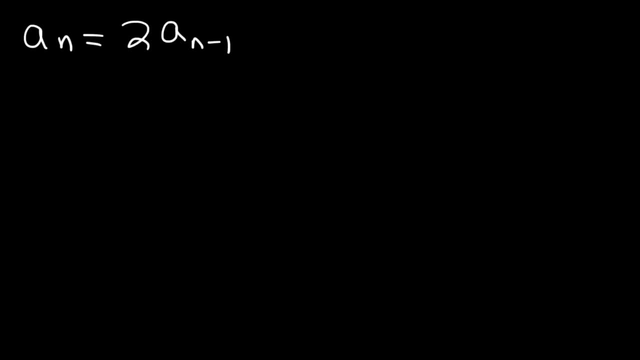 times a of n minus 1, and let's go ahead and square it and then we'll subtract it by 5.. So a of n plus 1 was the next term. a of n was the previous term. In this case a of n. 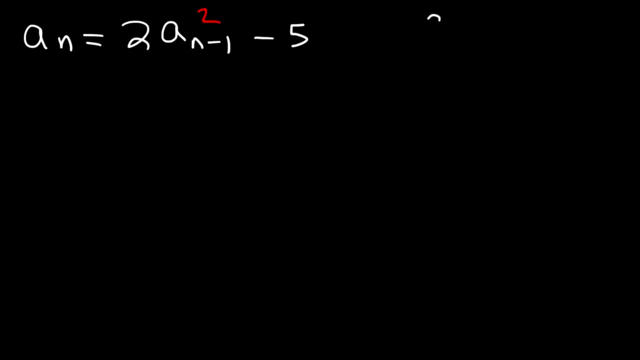 minus 1 is the previous term, a of n is the next term And let's say the first term is equal to 2.. So a of 2 is 2 times the square of a of 1 minus 5.. So it's 2. 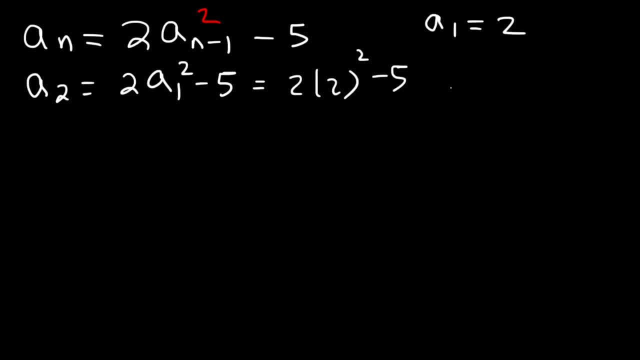 times 2 squared minus 5.. 2 squared is 4 times 2 is 8, minus 5, that's 3.. a of 3 is 2 times a of 2 squared minus 5.. So a of 2 is 3.. 3 squared is 9.. 2 times 9 is 18.. 18. 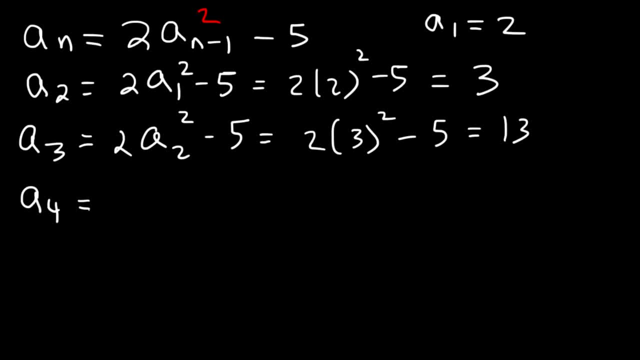 minus 5 is 13.. a sub 4 is 2 times the square of a sub 3 minus 5.. a sub 3 is 13.. 13 squared is 169.. 169 times 2,, that's 338 minus 5.. 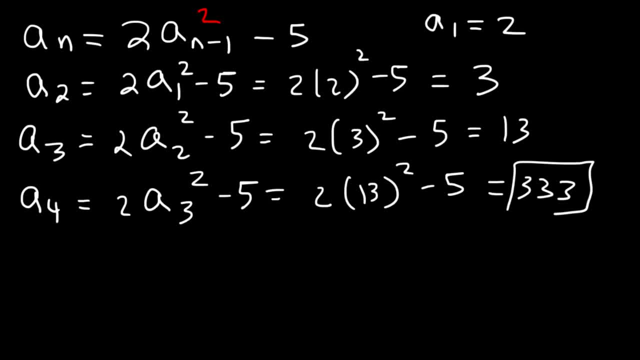 so this: this is equal to 333.. And so that's how you can work with a recursively defined formula.